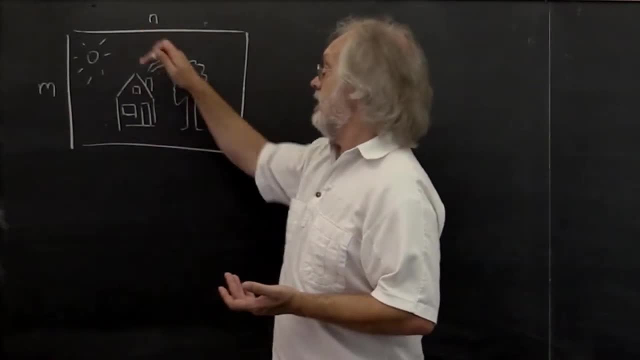 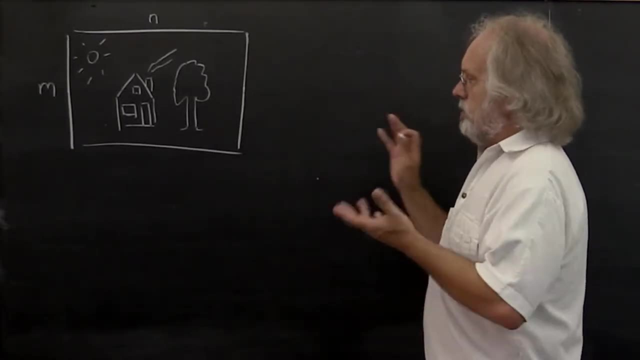 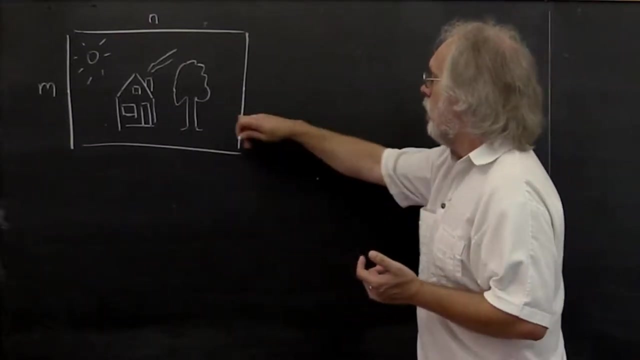 values. So we can think of it as an n by n matrix. Okay, so what if we don't want to store all of the pixels? What if we want to somehow do data compression? Well, if we call this the matrix B, then what we may want to do, 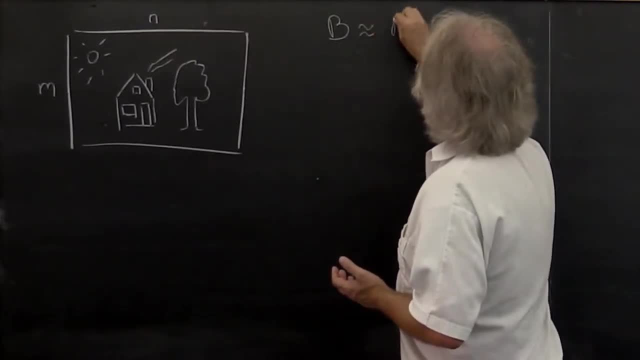 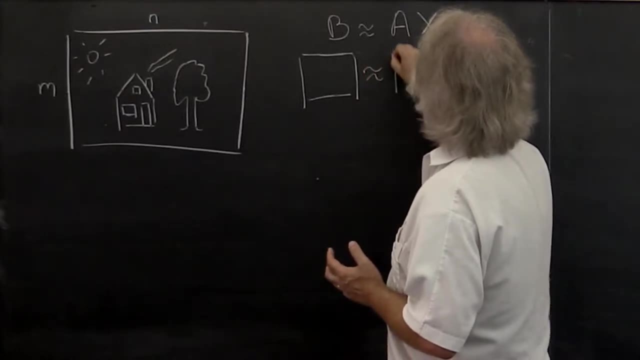 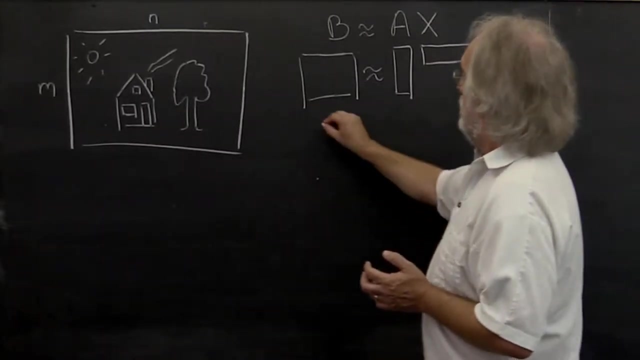 is approximate this with a matrix A times a matrix X, where the idea is that matrix B is the entire picture. A is a matrix with a matrix B. A matrix B is a matrix A with only a few columns And X is a matrix with only a few rows B. 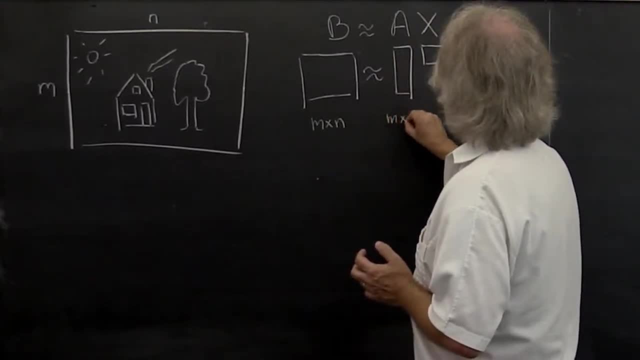 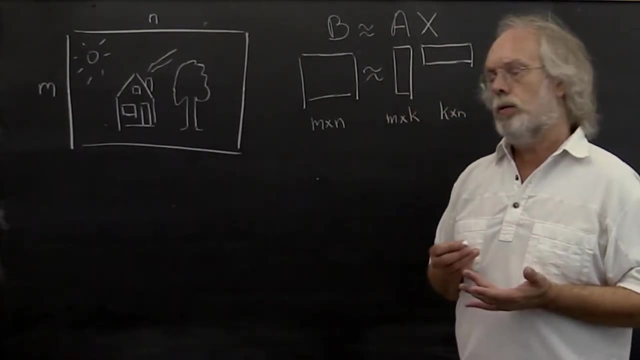 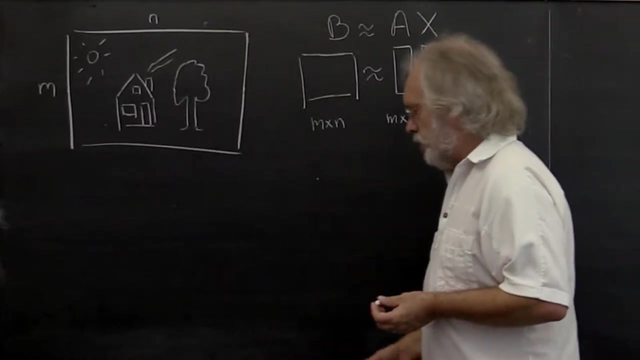 is n by n, A is n by k And X is k by n. All right, Well, how might we do this? Well, one way for coming up with matrix A could be to say: okay, we'll pick a couple of columns. 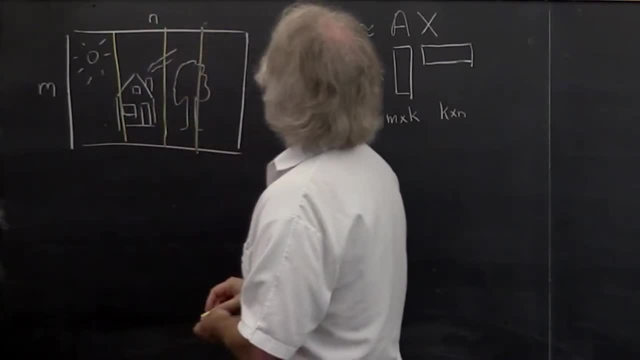 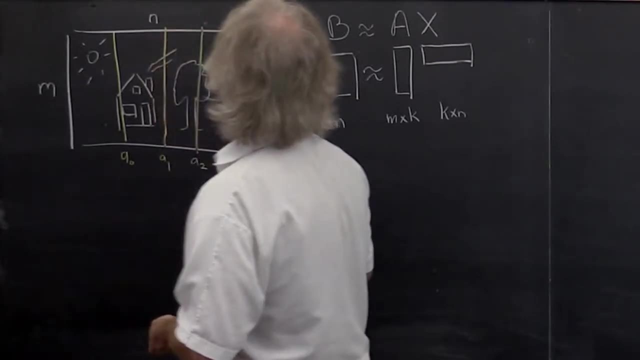 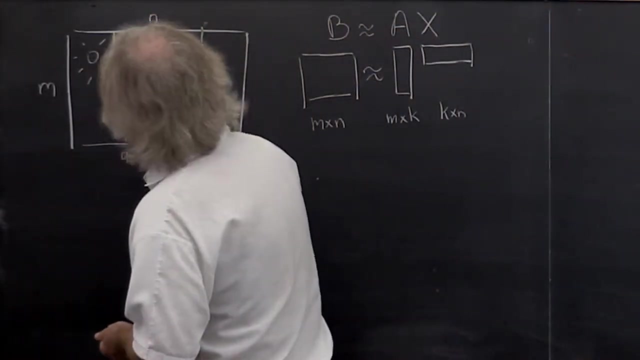 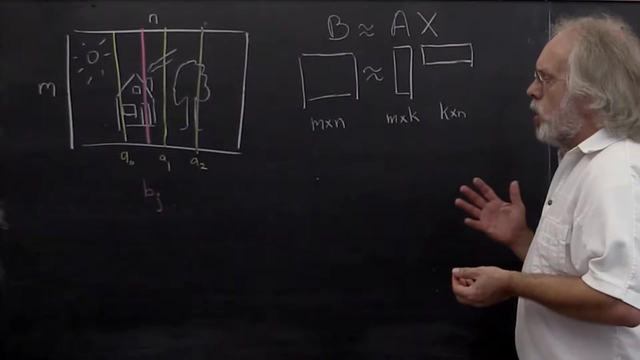 in our picture. Okay, Okay, Okay, Okay, Okay, And we'll make those, the columns in our matrix, A right. And then if we take an arbitrary column in our original picture, let's call it BJ. we're going to say, if 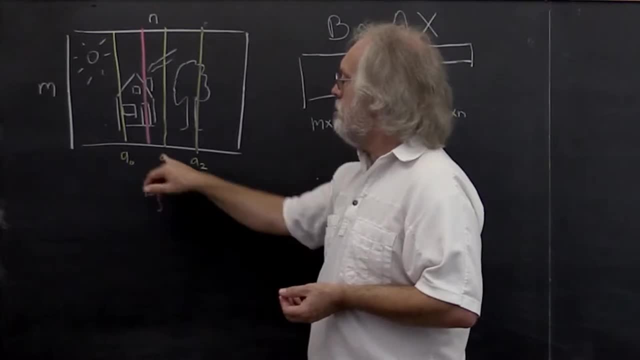 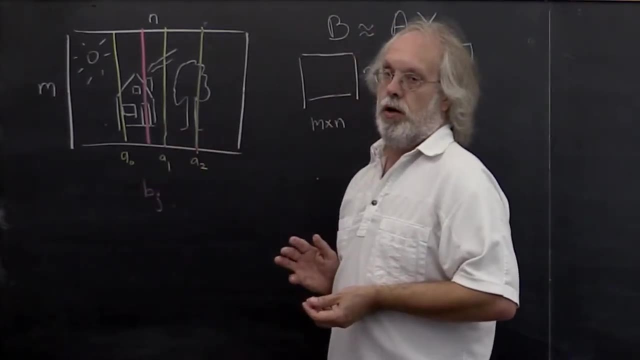 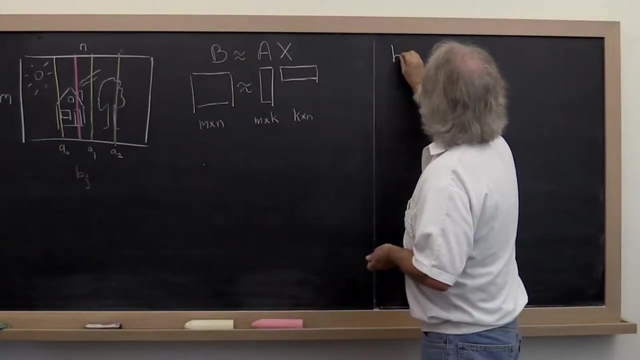 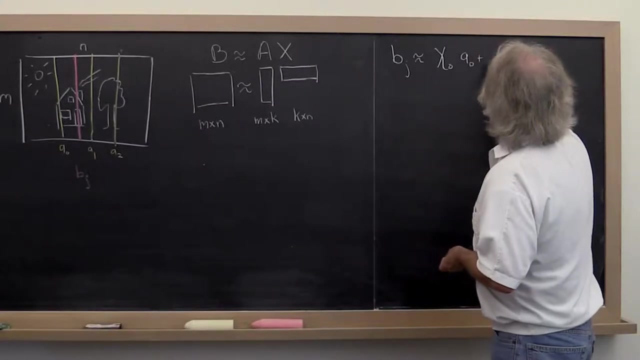 the columns that we picked represent the picture, then maybe we can approximate this column BJ as a linear combination of the columns that we picked for A. What does that mean? We're saying that maybe BJ is approximately some constant: chi 0 times A0 plus chi 1 times A1 plus chi 2 times A2.. 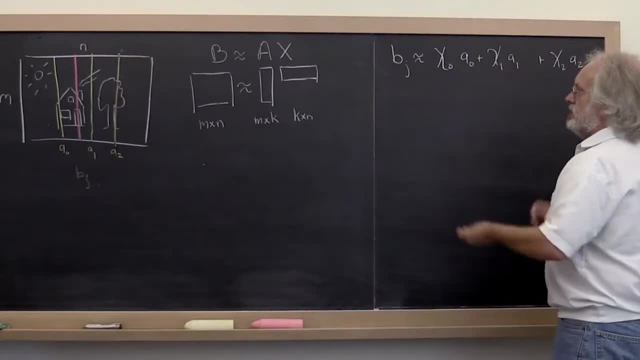 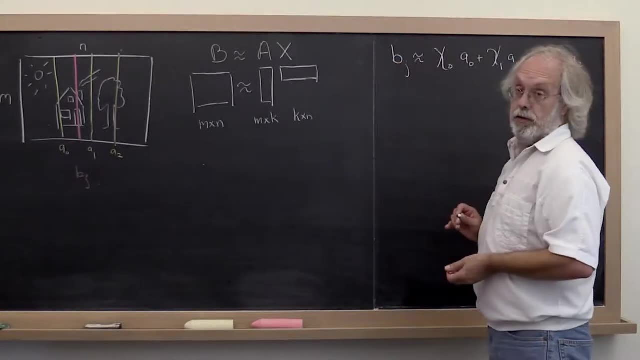 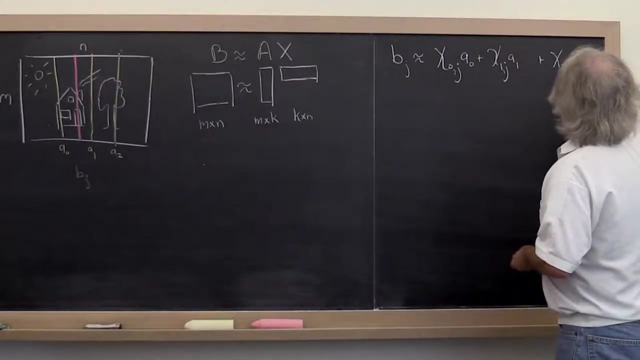 For the case where we pick three columns. obviously this generalizes to picking k columns. Now we're going to want to do this for every column of B, So we want to bring in a subscript j to indicate that these are the coefficients with which we take. 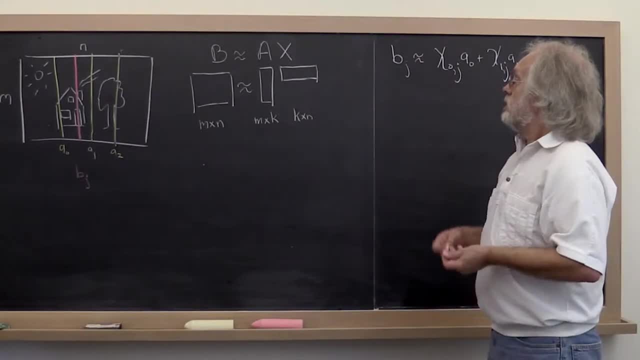 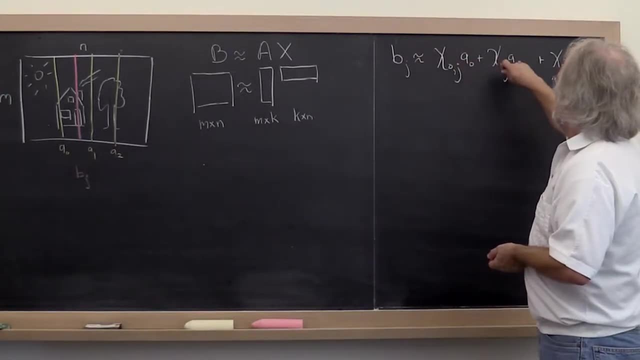 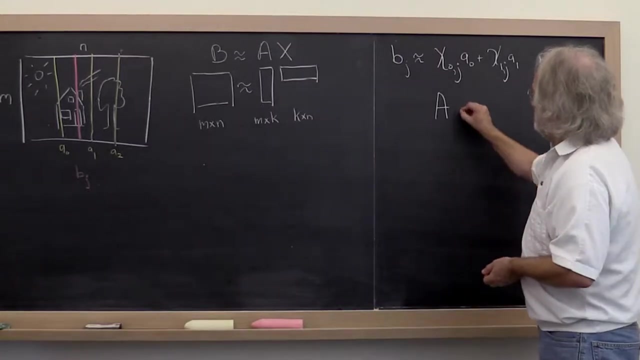 linear combinations in order to approximate the jth column of B. All right, Now we said: let's take A0,, A1, A2 to be the columns of A, So we can also think of this as A times xj, where xj is now the vector with entries. 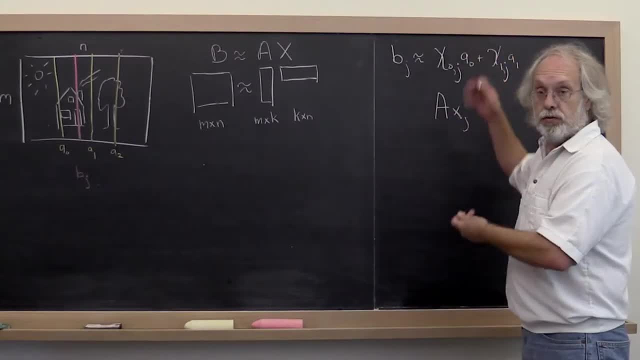 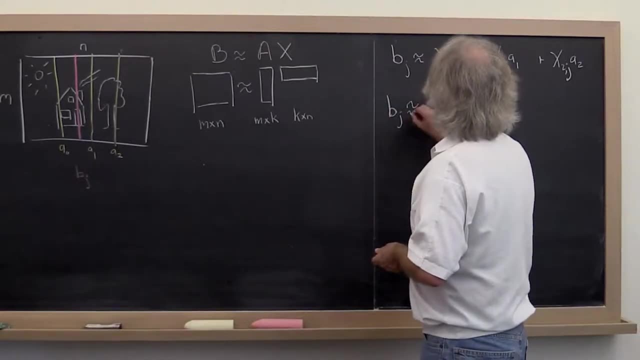 chi 0j, chi 0j, chi 2j or, in more general case, with k entries like that. So what we're saying is that BJ is approximately A times xj. Now we would like to pick our xj to be. 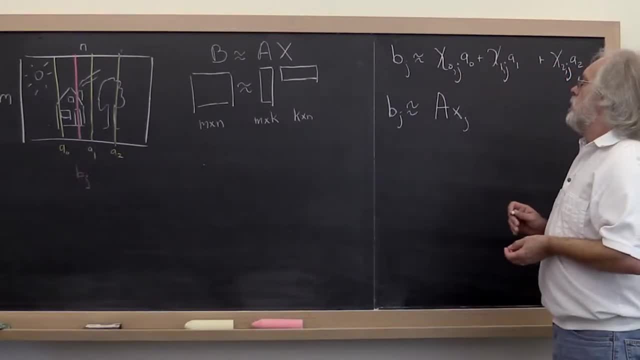 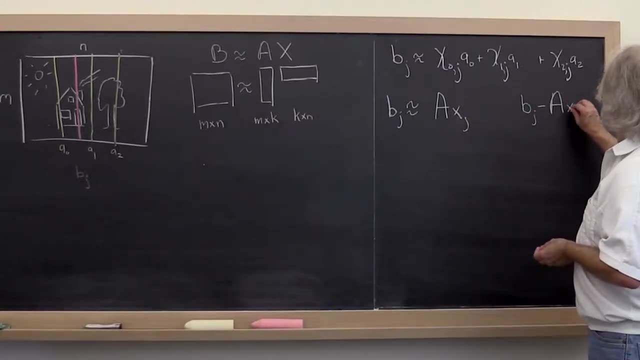 the best set of such coefficient? What is the best set of xj? All right, I'm going to write the box and the answer will be the question right here. So what we want to do is to take. What does that mean? Well, that means that we want to look at bj minus a times x. We 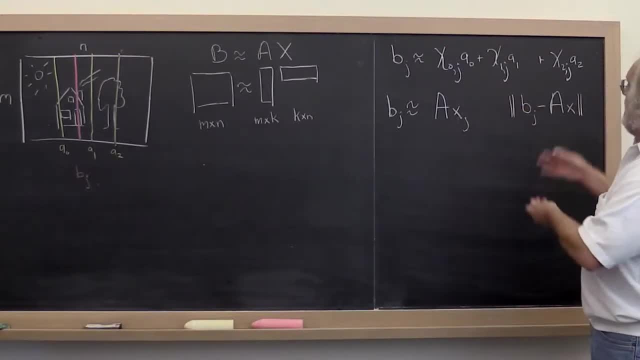 want to say: let's look at the magnitude of the difference. Well, we can use the two norm for the magnitude And then we can say: minimize that over all possible choices of x and pick your x sub j to be the vector x that minimizes all of that. 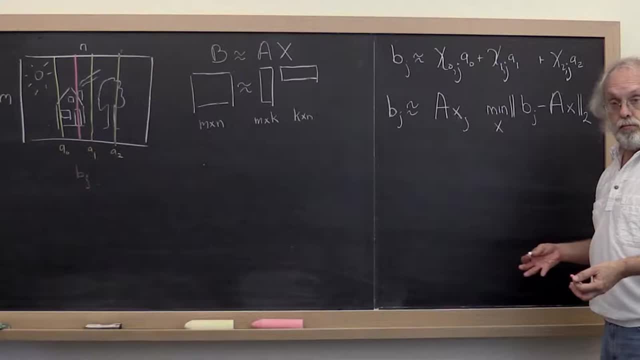 That's known as the linearly squares problem, Something that you saw in some linear algebra course at some point. It's something we'll delve into much more deeply later. if either you forgot or you didn't see Now, if A has linearly, 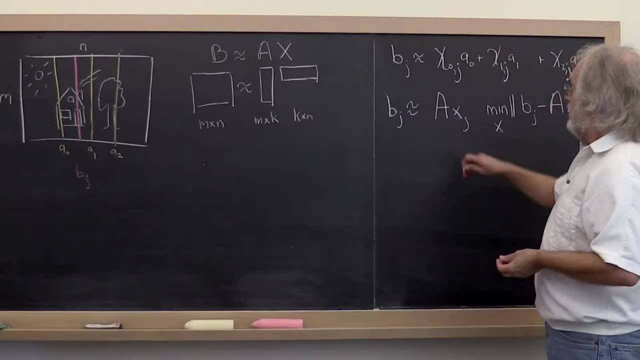 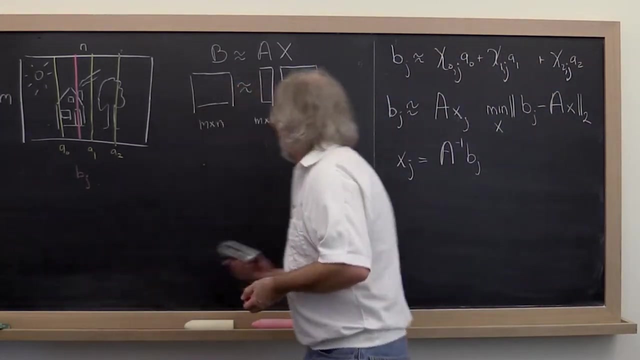 independent columns, then the best such solution is given by. well, let's see, if A were square and invertible, then xj would simply be a inverse times bj. right, But A has more rows than columns in this case, so we can't do that. Now there's something. 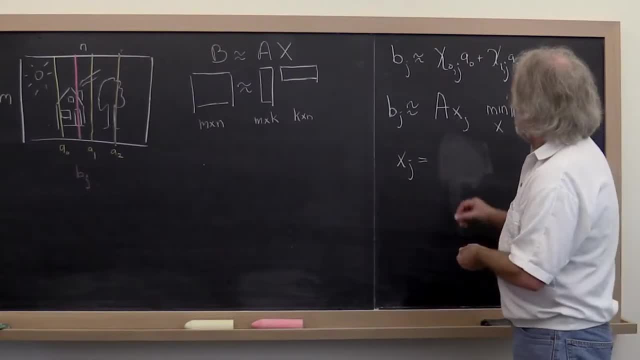 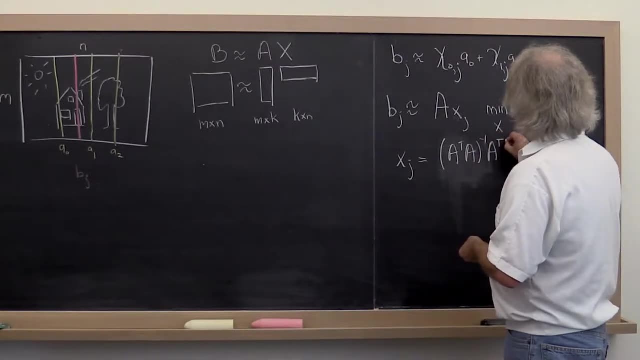 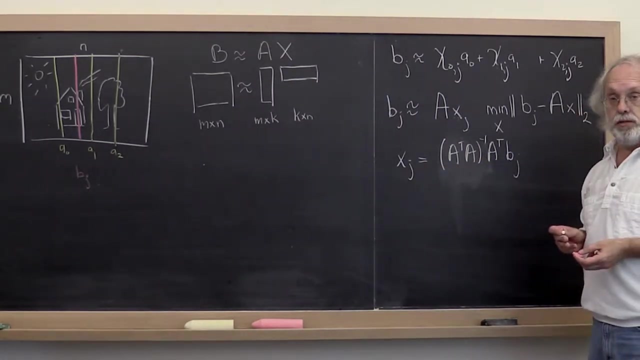 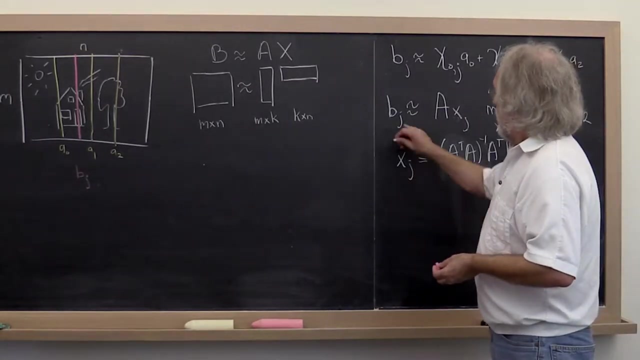 called the pseudo inverse. that takes its place, And the pseudo inverse is given by a transpose A inverse. A transpose times bj, And you can prove that this is the best choice. in the case where A has linearly independent columns, Alright. And what does that mean? Well, that means that our bj is approximately A times that vector. 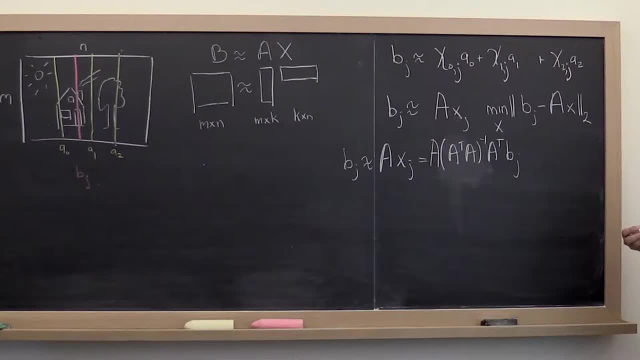 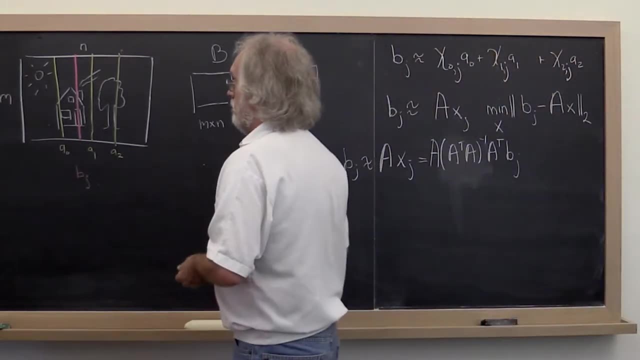 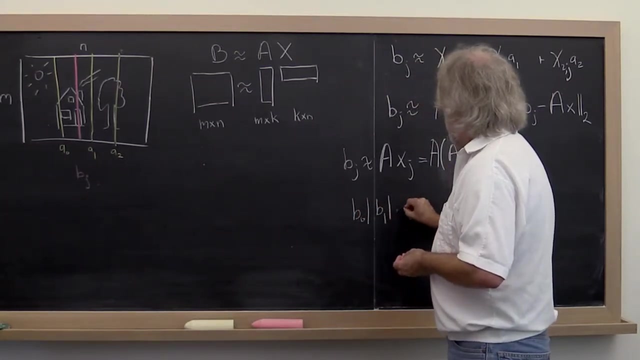 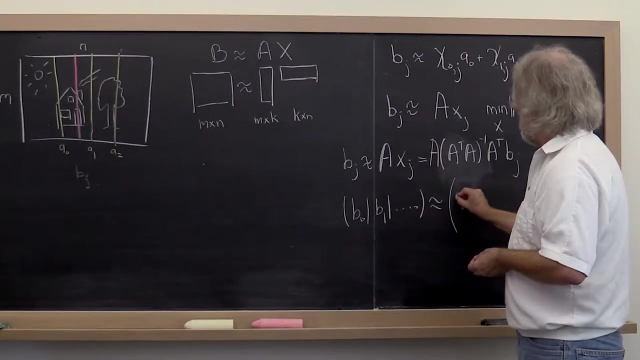 which is given by that right there. Now, what if we do that for all of our columns in our picture? Then we would say: okay, b0,, b1, and so forth is approximately equal to: let's see, the first column would be approximated by: 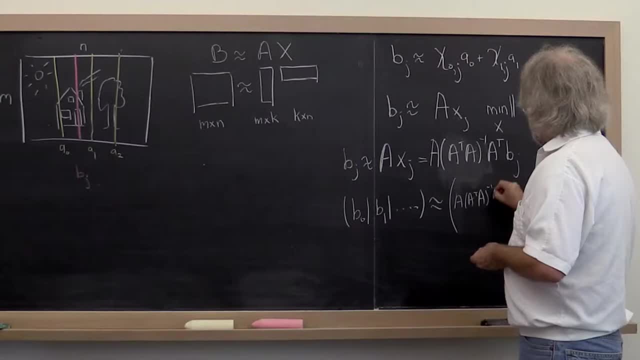 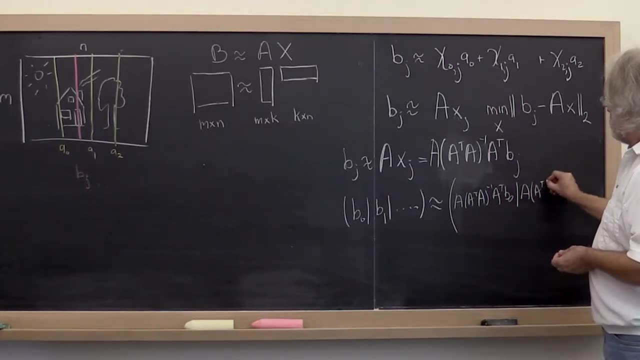 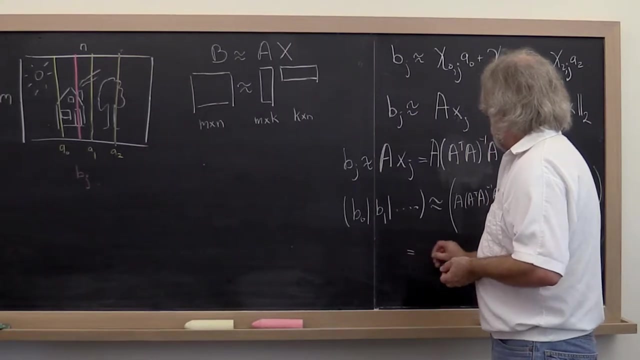 A. A transpose A. inverse A transpose bj. The second column would be approximated by A times A transpose A. inverse A transpose b1, and so forth, And you should recognize the fact that we can then bring this matrix out And this is actually equal to A times A transpose A. 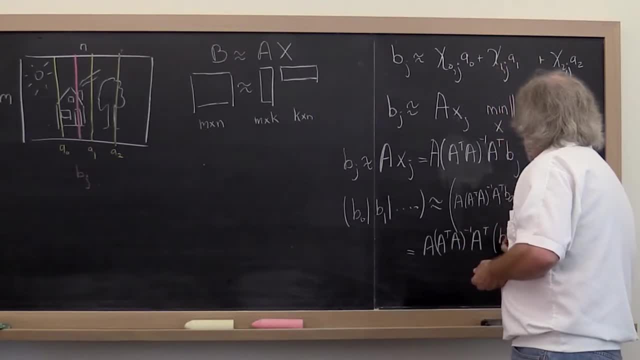 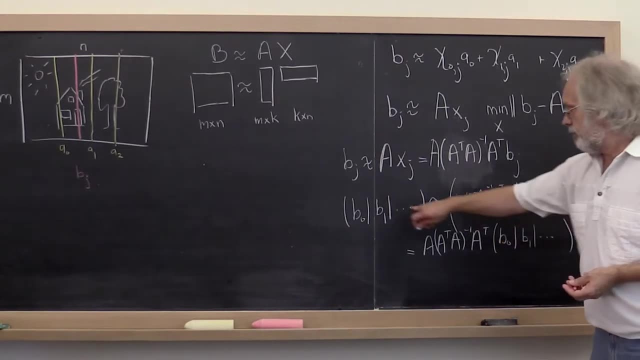 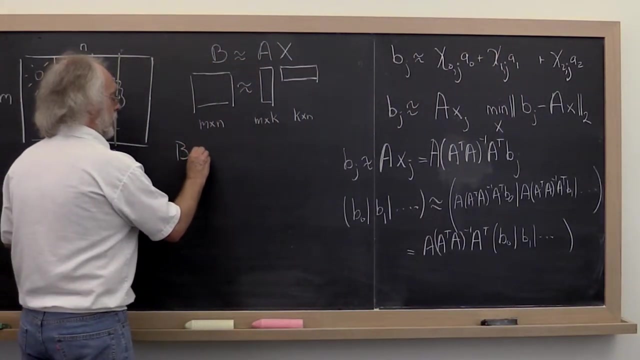 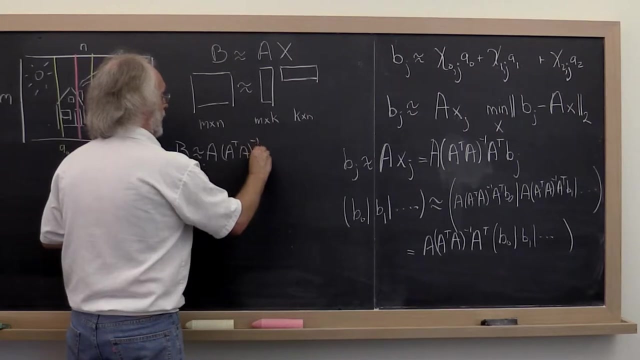 inverse A transpose times b0,, b1, and so forth. This is equal to that and therefore this is approximately equal to that. So what do we have now? We have that b is approximately equal to A times A transpose A. inverse A transpose times b. 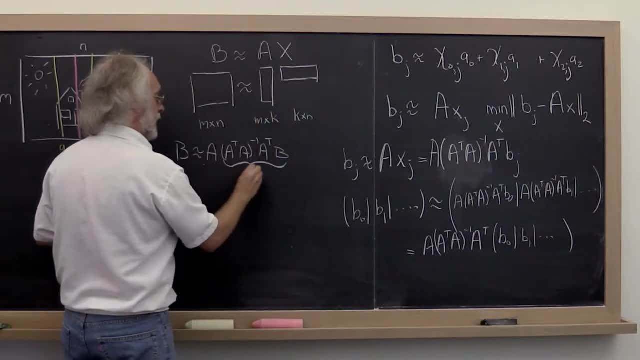 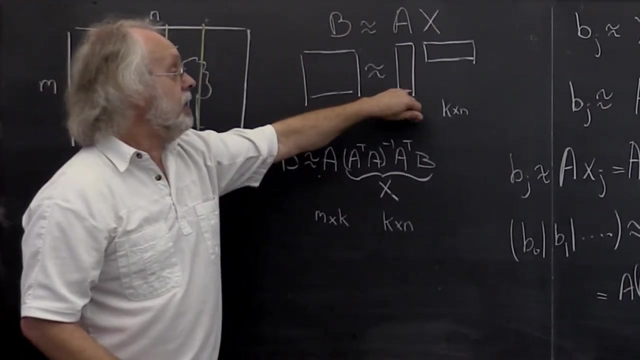 We can choose this to be our matrix X. This matrix is then m by k. in general, This matrix you can check is k by m, And what we have now is a formula for computing a rank-k approximation to our picture. You can check that this is a. 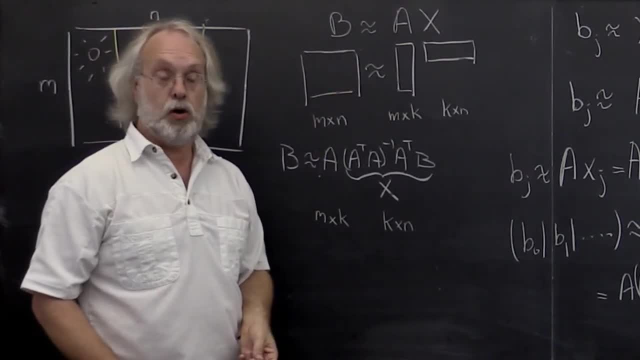 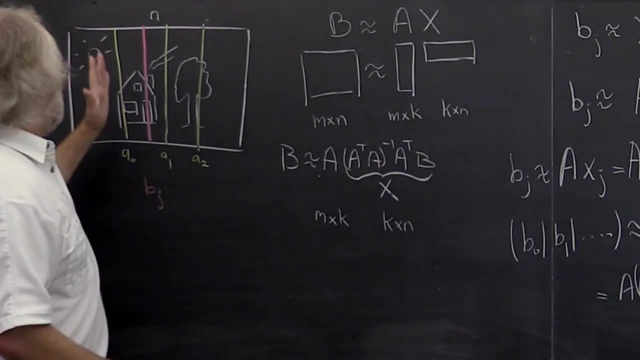 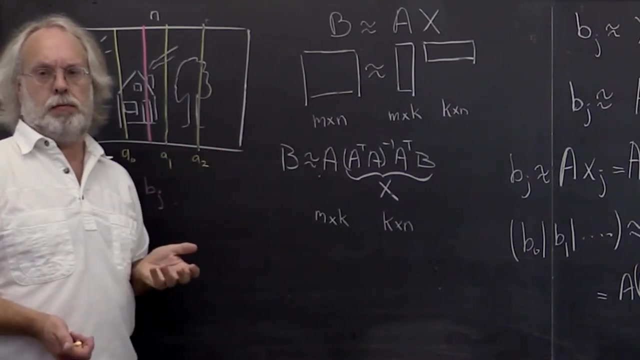 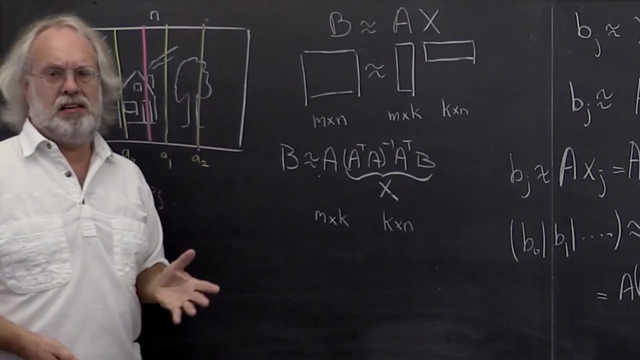 rank-k matrix: Alright, Now you can say: well, it would seem to me that there must be optimal columns in my picture, Then I can pick to get the best approximation. And then you might say: well, it would seem like how many columns I pick would influence how accurate of